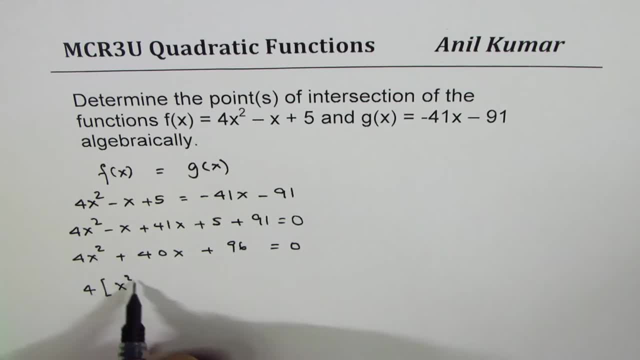 out 4, which is a common factor. So we get x square plus 10x 4 times 2 is 8, and then 4, 16, equals to 0.. Now, inside we're looking for a product of: 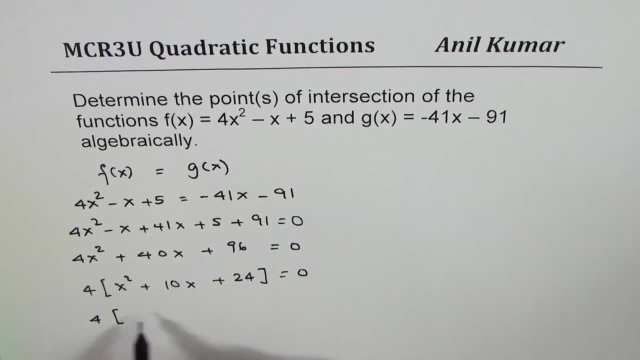 24, sum of 10, which is 6 times 4, right. So we could write this as: x plus 6 times x plus 4, right equals to 0. So that gives us 2 points. x plus 6 equals to 0, that means x equals to. 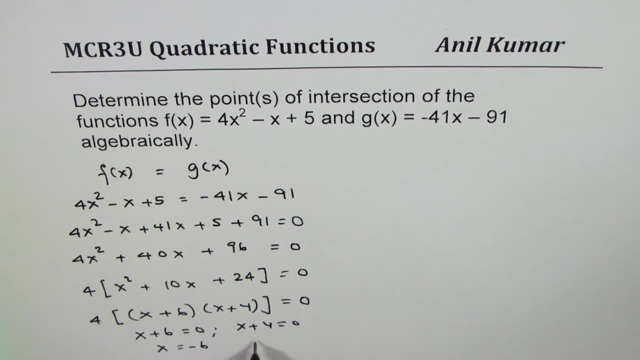 minus 6, and x plus 4 equals to 0 gives x equals to minus 4, correct. Now we got the x coordinates, we have to find the y coordinates also, so don't forget that right Now you could use any one of these equations to find the y coordinates When x equals to minus 6,. 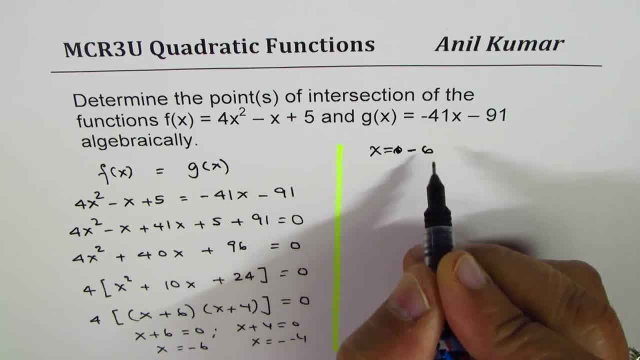 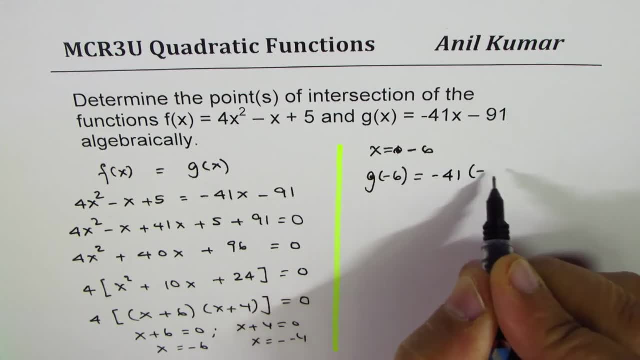 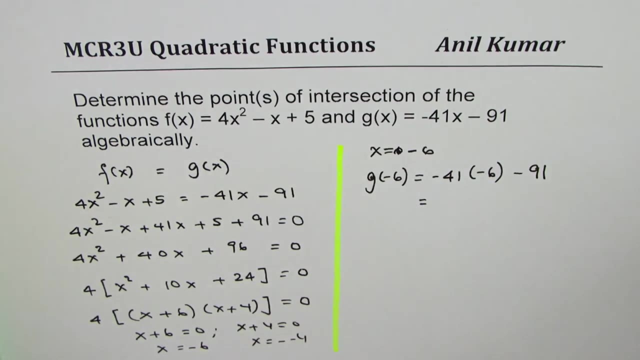 I mean, okay, when x equals to minus 6, we can find g of minus 6 as equals to. we'll place it here, right, Minus 41 times minus 6, minus 91, correct. So that gives you- let's use calculator, okay, Minus minus is positive, so I'll just 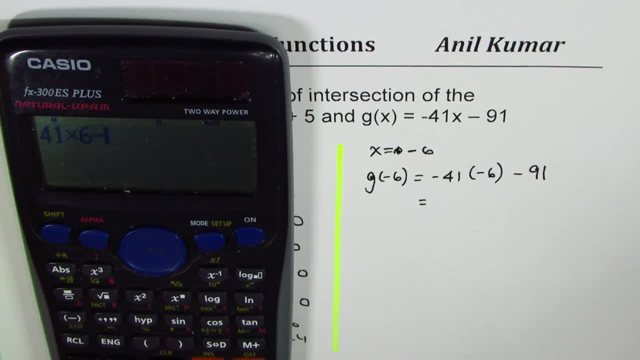 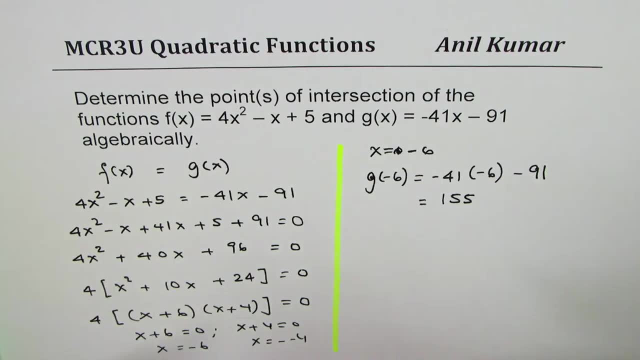 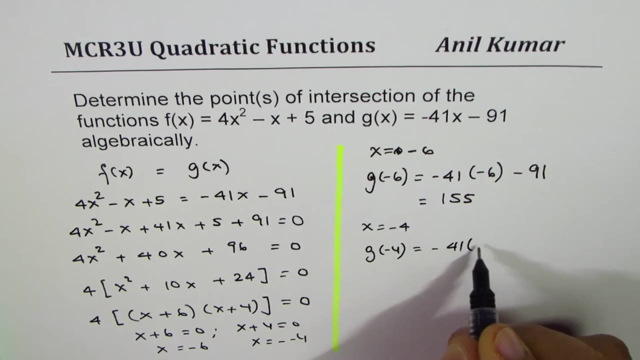 do 41 times 6, and then take away 91, and that is 155.. The other value is x equals to minus 4,. that means we can calculate g minus 4, which is minus 41 times minus 4, minus 91,. 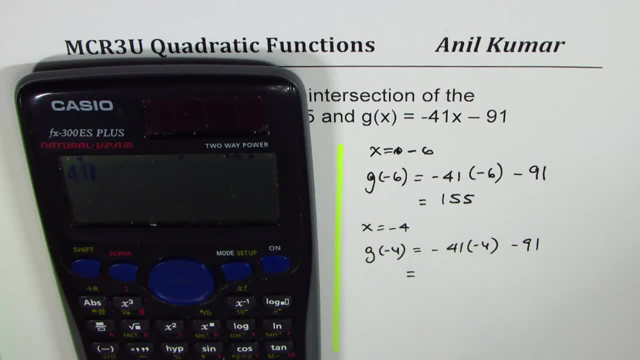 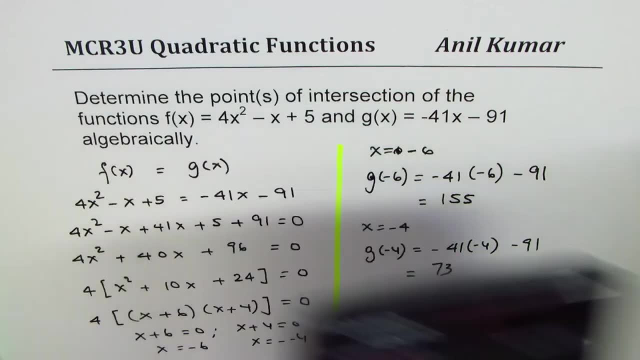 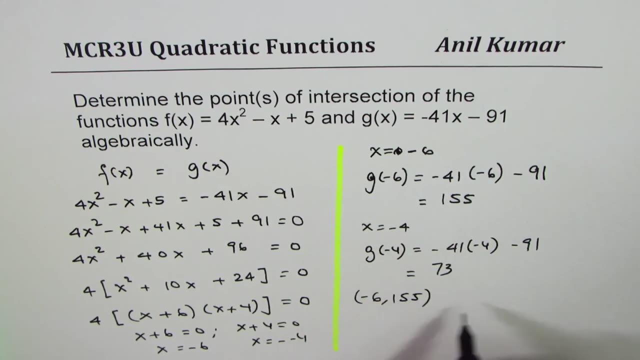 and that is equal to. so this time we'll do 41 times 4, and then take away 91, right 73.. So that gives you coordinates of 2 points, and these are minus 6, 155, and minus 4, 73,. 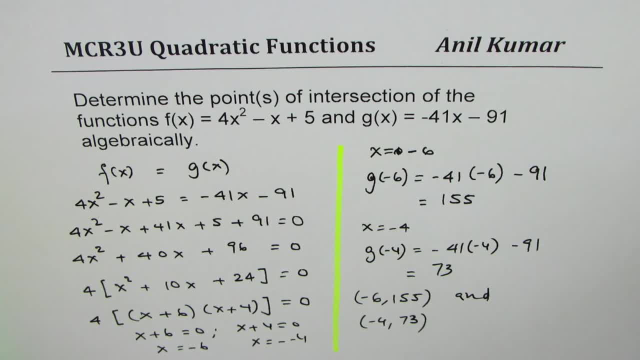 right, So that becomes the answer for the given question. I hope it is straightforward. Feel free to post your comments. share my videos. Thanks for watching.